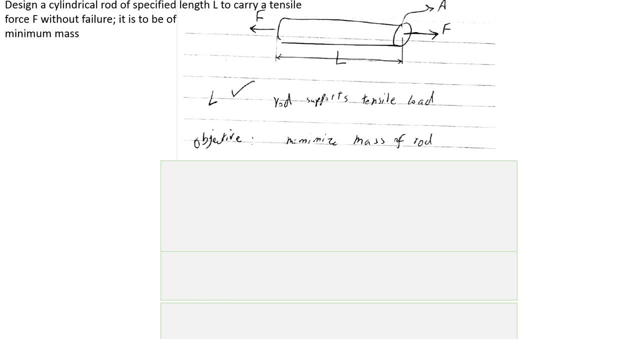 Of course we have three variables, which is area and type of material that we want to select it from the list, The list that we have in the CES software. Here maximizing the performance is actually minimizing the mass, while still the rod can carry the load F safely without failure. 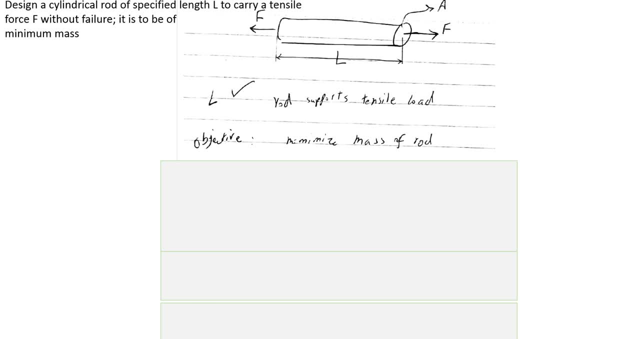 Thank you for watching. Next step is to find an equation or relation for the function or for the quantity that you want to maximize or minimize it, And that's, of course here is mass. Mass is related to area length and density, as you can see here. 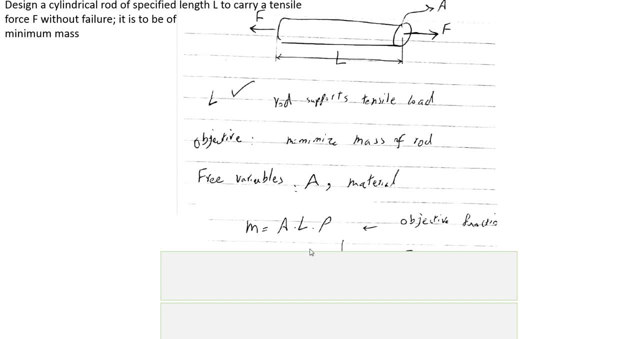 And, as we said, three variables are: A and materials. This is our objective function. We want to minimize this function. At the same time, we want to make sure that this function is satisfied. We want to make sure that this rod withstands the tensile load of F. 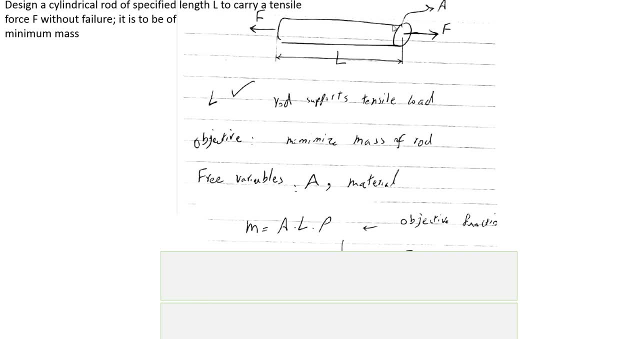 So the stress in this cross-section, in different cross-sections of the rod, should be smaller than the failure strength of the material. That's what we show here. So F over A, which is the stress, should be smaller than the failure strength. 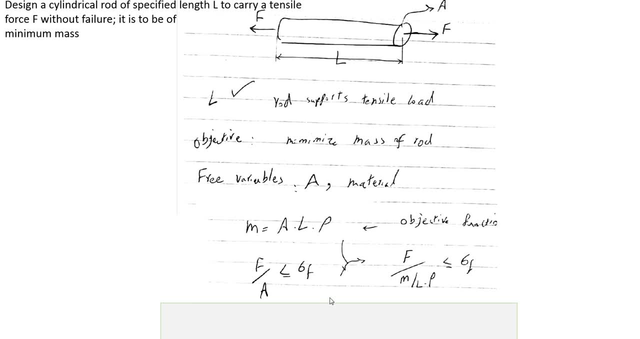 If you combine this and remove the stress And remove parameter A from these two relations, We end up to this relation, the new relation that you can see: Force divided by mass over length times. density should be smaller than sigma F. If we flip this fraction then we will have M over L, rho F is bigger than 1 over sigma F. 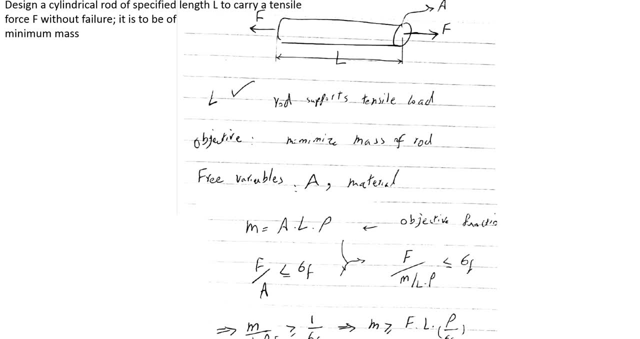 Or finally, M is bigger or equal than this relation. here F is force length. density over sigma F over failure strength. Here the last bracket contains the material properties. Of course the lightest rod that can carry force F safely is the one that is made of the material with the smallest value of rho over sigma F. 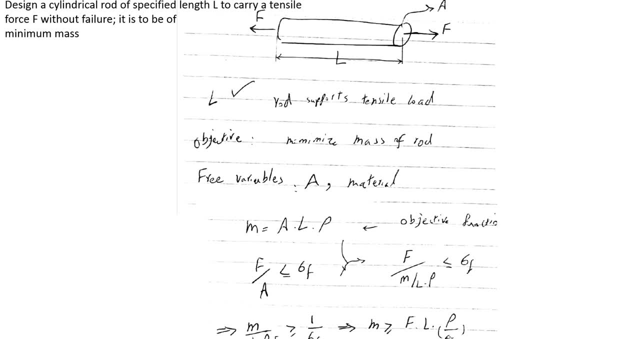 In other words, minimizing density over failure strength results in minimizing the mass. So density over failure strength can be our material index. But because usually it's easier to talk about maximizing, Then we introduce our material index as the inverse of this relation. So here material index is going to be failure strength divided by density. 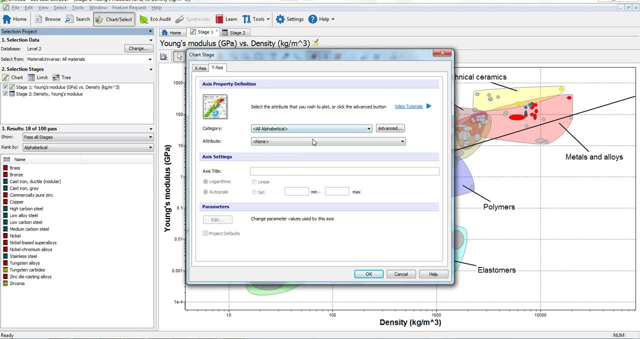 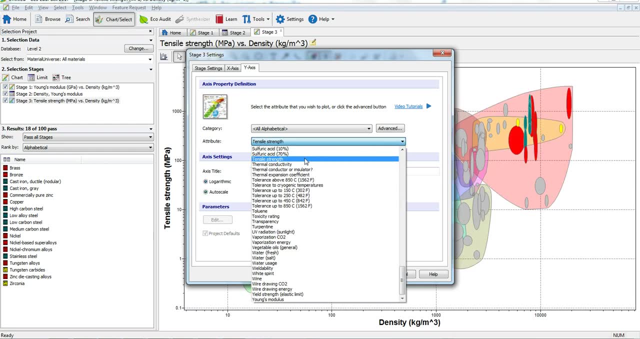 And our goal is to maximize it. Let's go to the chart, again, to the CS chart. On the Y axis we have failure strength, Which from this menu we choose tensile strength, And on the X axis we have density. 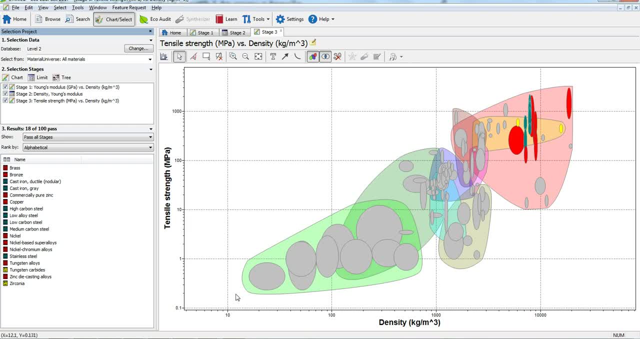 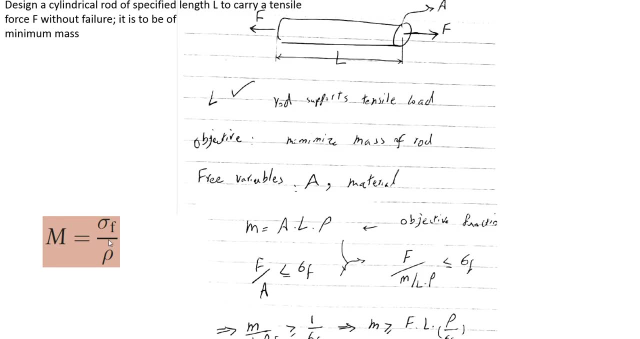 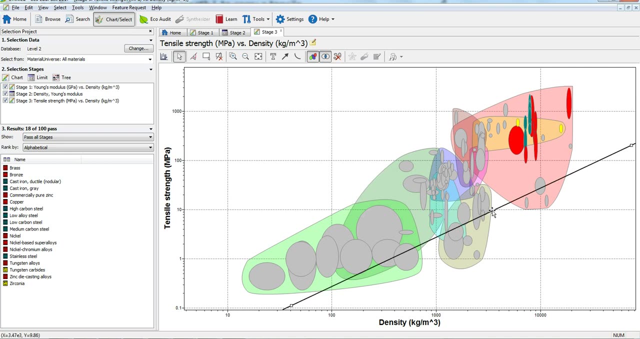 We press OK, Now we have different types of material And because our goal is to maximize strength by density. So what we do and the order is 1.. So we draw a line that has Slope of 1. And we insert it anywhere in the tensile strength versus density chart. 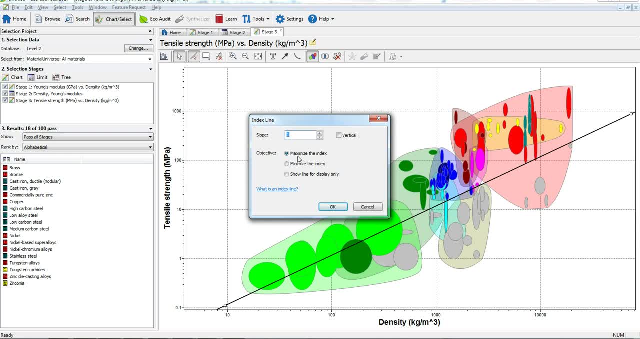 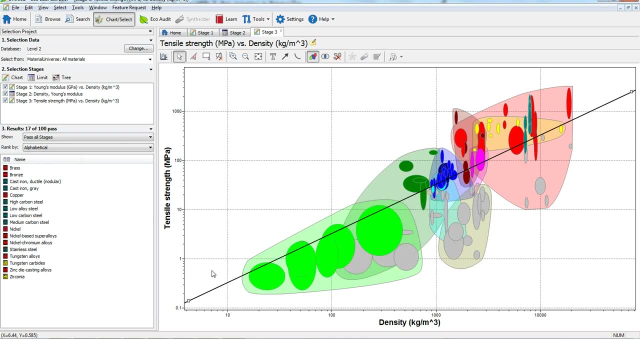 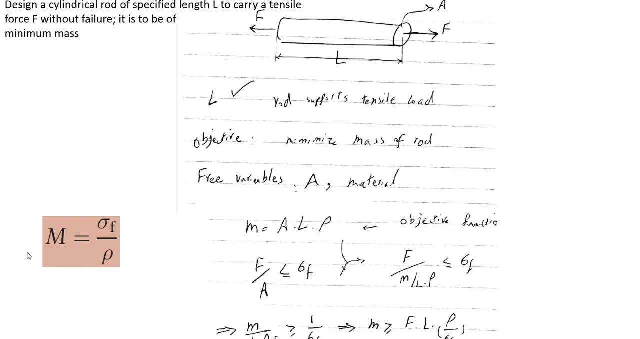 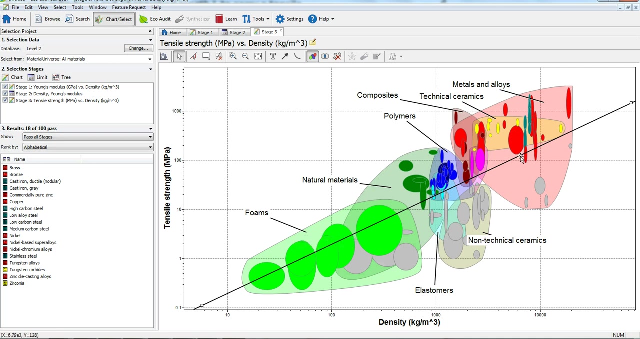 Look, because we here stated that we want to maximize the index, So any material above this line is accepted And the line shows loose material. Loose sigma F Over rho is equal to 1.. Sorry, my mistake. They have the same value of material index. 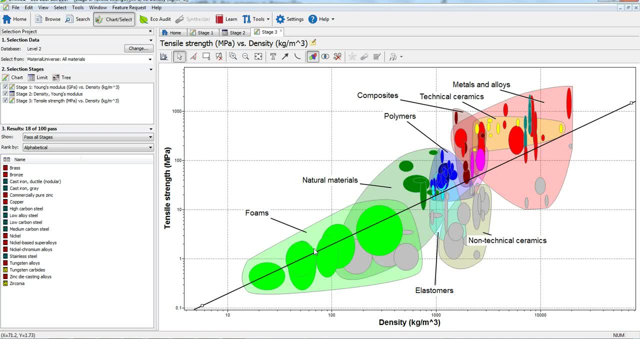 Which is tensile strength over density. Every material on this line, And you see, by going to the left We remove more material from the selection And this material is left in the list If you want to maximize sigma F over rho. Of course, the last two groups of material that are left are metals and composites. 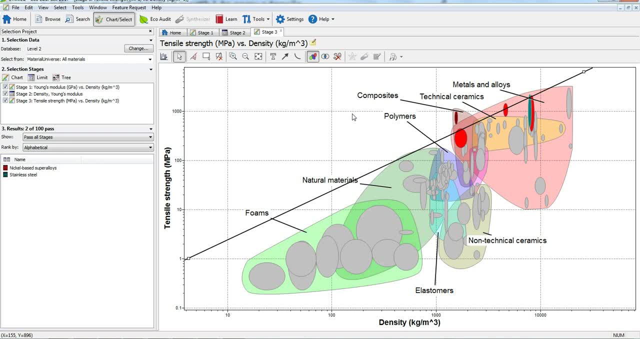 If we have further limiting or limiting properties, Like what we had in the previous video, Then we can of course have a smaller range of material to select from. Thank you,